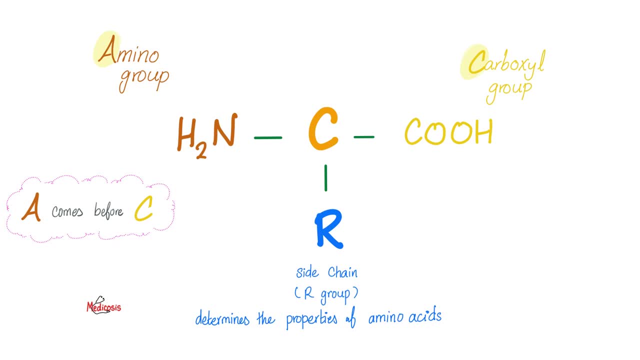 amino acid. you have an amino group here. So if you have an amino acid, you have an amino group here. Chemical properties, that is. Does the order matter? Like: should I write the amino here or here? Like, does it matter Amino first or carboxyl first? Yes, of course it matters. A comes before. 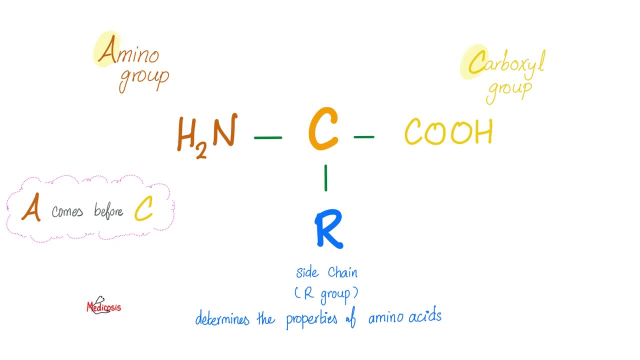 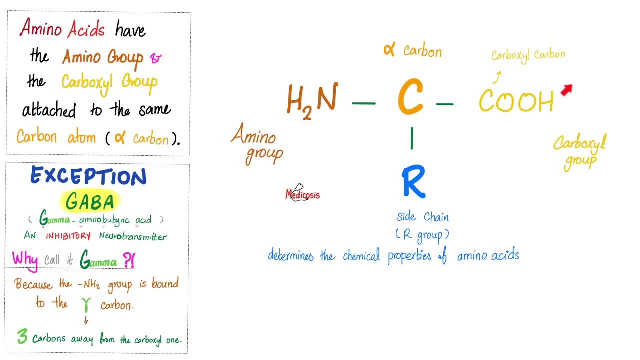 C in English, right Yep, amino groups comes before the carboxyl group. What's the name of that carbon? Alpha carbon. Here's the beauty of the amino acids: They have their amino group and their carboxyl group attached to the same freaking carbon known as the alpha carbon. 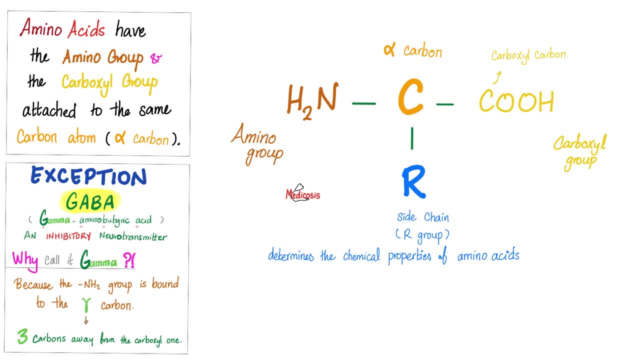 Is there an exception? Of course, every rule has exceptions. This is GABA. GABA stands for what? Gamma Amino Butyric Acid. Say it one more time, because it was so beautiful: Gamma Amino Butyric Acid, Gamma. You know why we call it gamma? Yup, indeed, Because 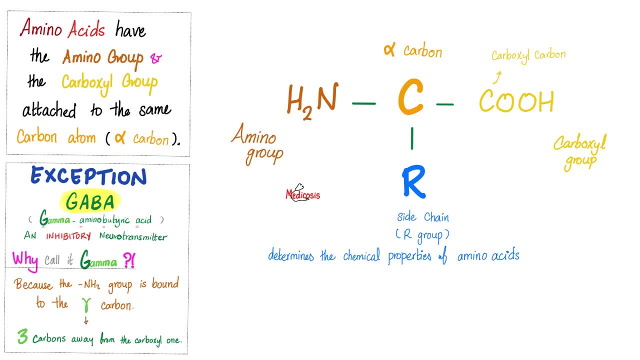 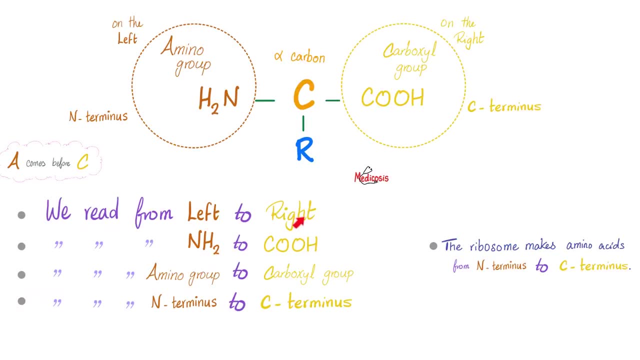 it's a gamma carbon which is three carbons away from the carboxyl one. So after the carboxyl you have alpha and then you have beta and then you have gamma carbon. In English we read from left to right. Same thing with amino acids. We read from the amino group towards the carboxyl. 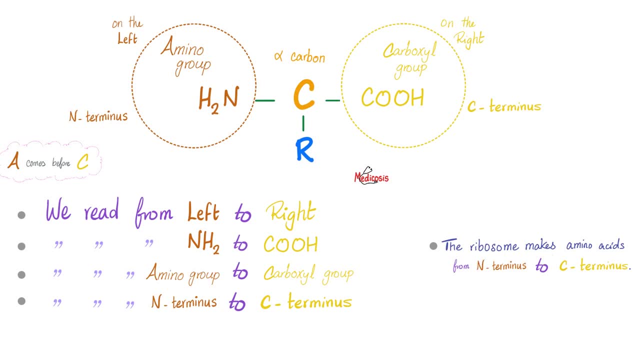 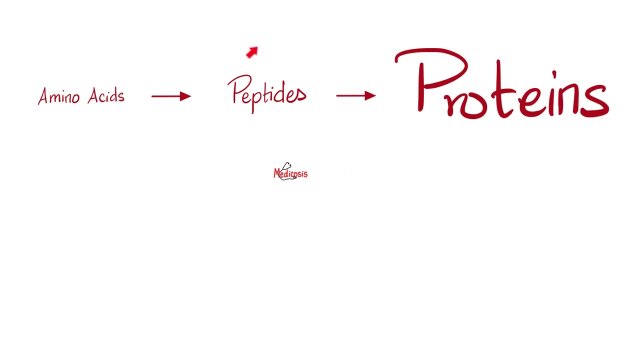 group. Why do we care? Because this is the order of the amino acid coming out of the freaking ribosome on the rough endoplasmic reticulum. if you remember, The ribosome makes the N-terminus first, before the C-terminus. That's why we care. Here are amino acids. They become peptides. 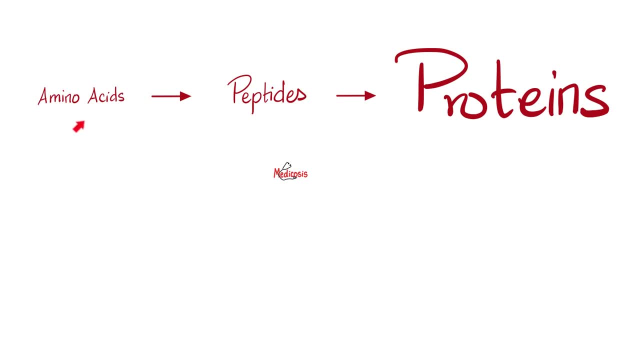 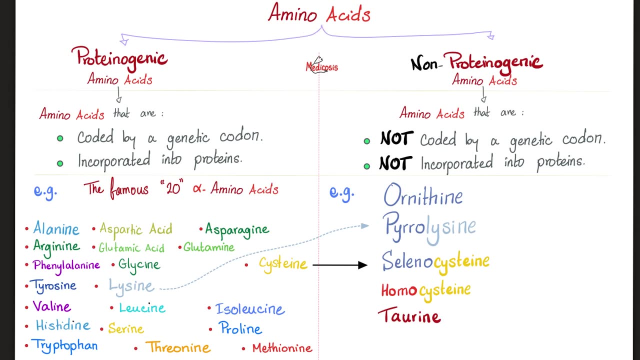 and then they become proteins. These are the macromolecules. These are the micromolecules, Polymers, Monomers. Let me ask you a question: How many amino acids do we have in our bodies? Oh, I know No. medicosis, My biology professor, told me that we have 20 amino acids only. 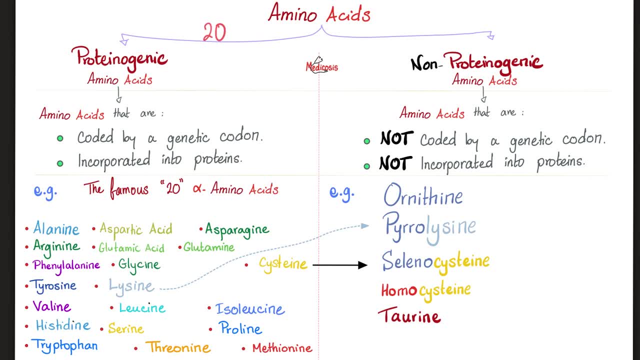 Shut up. Your biology professor is myopic. No pun intended. The 20 amino acids that you're talking about are only the proteogenic amino acids. You have other non-proteogenic amino acids in your freaking body, But what's the difference? Proteogenic amino acid just by. 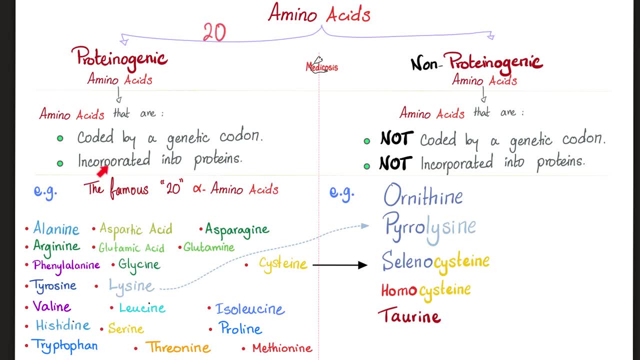 the name. Look at the name: Proteogenic, So they will make proteins. Oh yeah, They are incorporated into proteins. Amino acid, an amino acid, another amino acid. make them into peptides and then proteins. They are also coded by a genetic codon. Remember these three lovely nitrogenous bases? What are 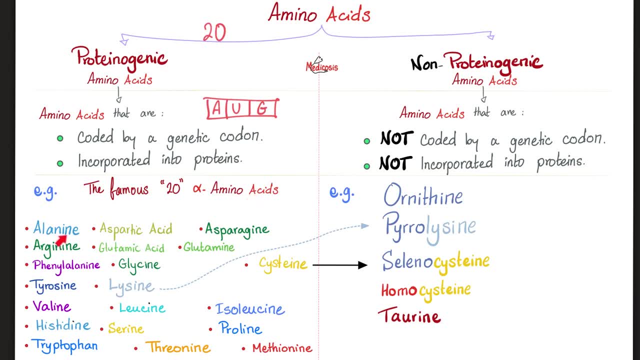 these 20 amino acids that your biology professor told you about? Yeah, the famous alanine, aspartic acid, asparagine, arginine, glutamic acid, glutamine. So you have aspartic acid, asparagine. 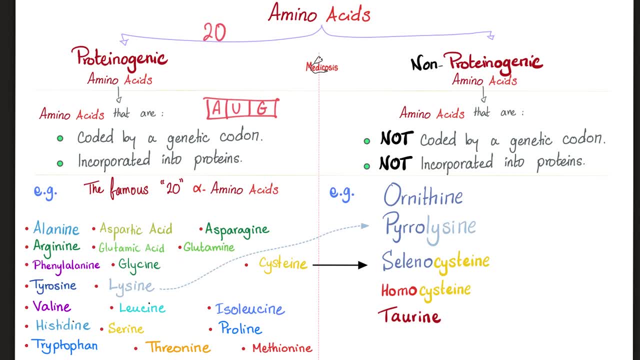 glutamic acid, glutamine, phenylalanine, glycine, tyrosine, lysine, valine, leucine, isoleucine. You need to remember these three together: Hyaline, leucine, isoleucine, histidine, cysteine, serine, proline, tryptophan, threonine, methine. 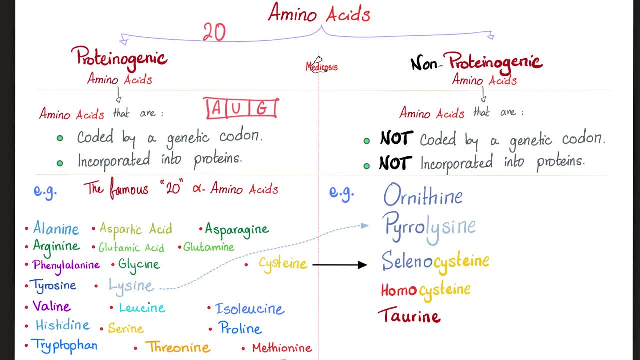 My favorite, Because it gives your Uncle Sam a methyl donor. How about the non-proteogenic? All right, They are not coded by a codon, They are not incorporated into proteins, But they exist, such as ornithine, If you remember your urea. 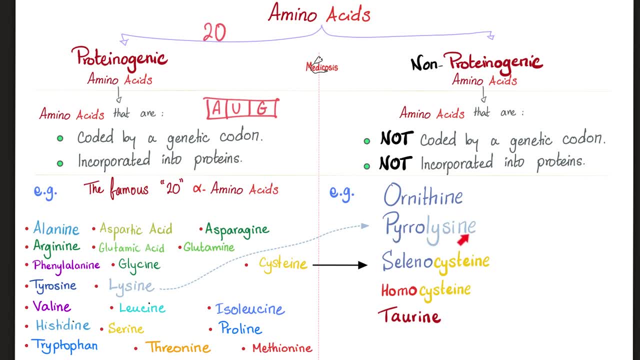 cycle Pyrolysin. Where the flip. did you get pyrolysin from? From lysine Selenocysteine. Where do you get it from? From cysteine? Selen means selenium Pyro because it contains pyruline ring or pyruline side chain. Where did homocysteine come from From? 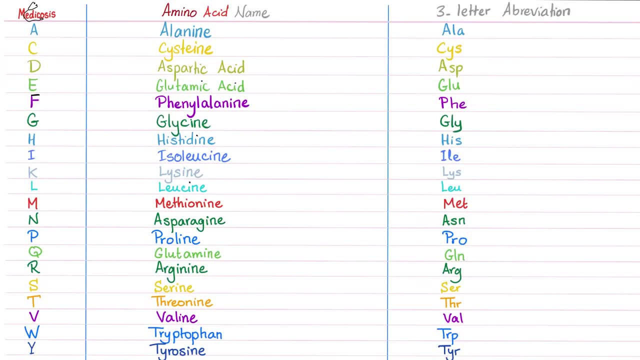 cysteine. Do you remember the coagulation factors? Yeah, Each one had a name and a number. Okay, Amino acids: Each one has a name, a one-letter abbreviation and a three-letter abbreviation. You need to memorize all of this. 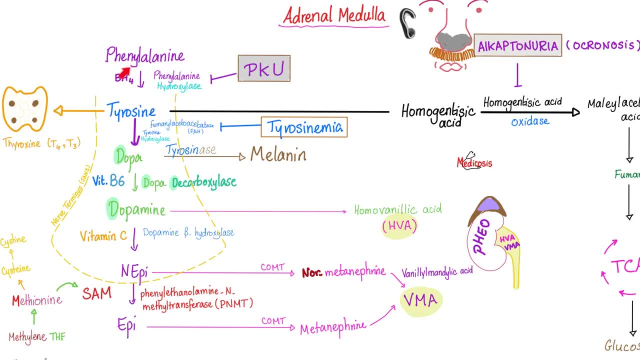 Do you remember this? Do you remember the story of the adrenal medulla Sure? Phenylalanine, tyrosine, dopadopamine, norepinephrine, epinephrine- You see that That is Sam. Where did Sam come from? Methionine? 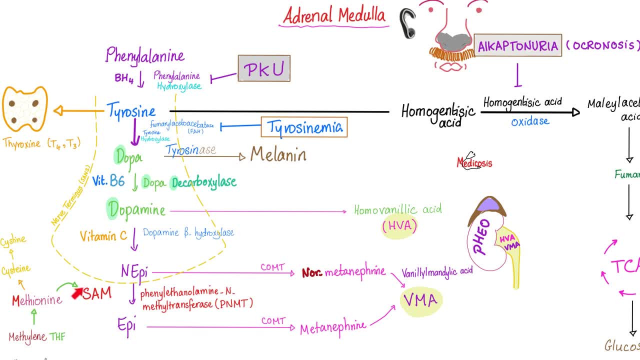 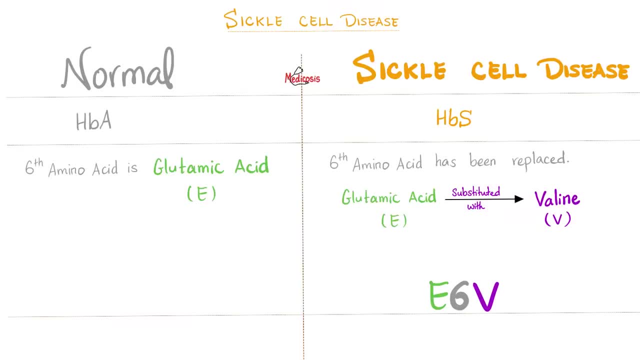 What is Sam, A methyl group donor? Where did it get the methyl group? From methionine, Because methionine contains methyl. it also contains sulfur. Now that you know the abbreviations, let's talk about sickle cell disease. All right, 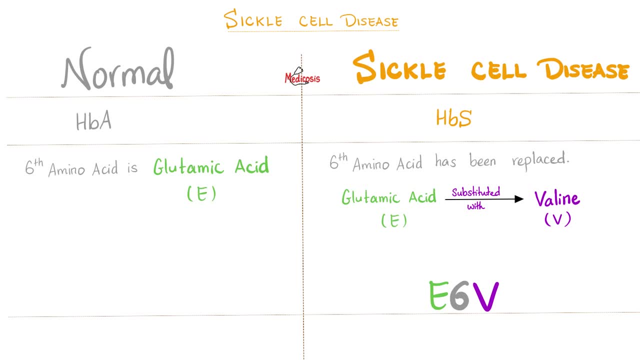 How do you differentiate between a normal person and a person suffering from sickle cell disease? Normal person: have hemoglobin A. Sickle cell disease have hemoglobin S. Why do you call it A? A for adult? That's the normal hemoglobin in adults. How about hemoglobin S? This is for 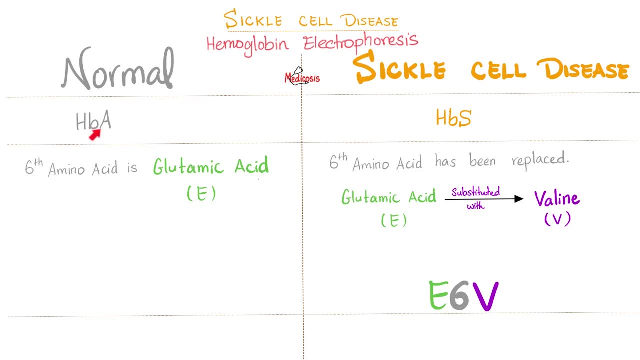 sickle cell. How about the fetal hemoglobin? It's going to be called hemoglobin F, F for fetus, But if Gordon Ramsay were your teacher, F will stand for F me. Normally, as you know, hemoglobin is made of what Heme and globin, And heme is made of what Hemoglobin And hemoglobin is made of what 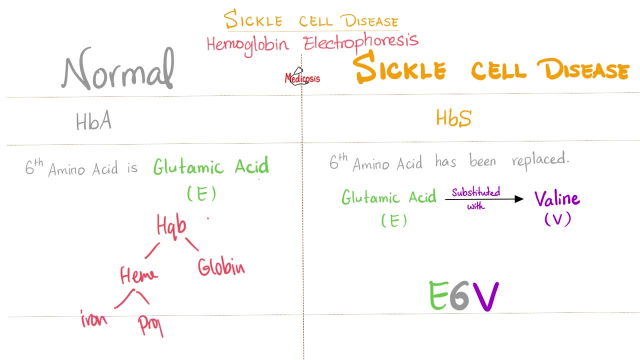 Iron and protoporphyrin And globin is made of what Amino acids? All right, Tell me about these amino acids. Number six should be glutamic acid. That's normal, But in sickle cell disease the glutamic acid has been substituted with valine, And that's abnormal. We should have 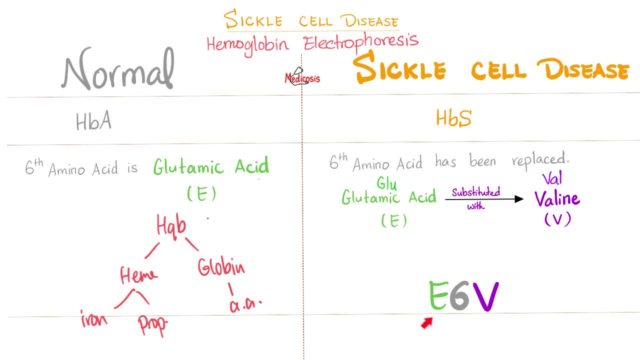 glutamic acid. Oops, Now we have valine, So we call it this E6V. What the flip is that Normally I should have E at position number six. Unfortunately, now I have V. So when you say E6V, I know that you're talking about sickle cell. 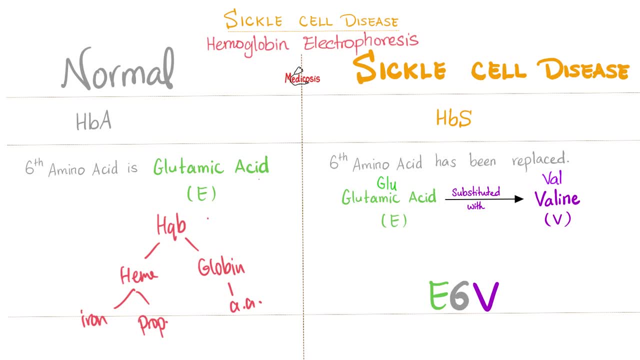 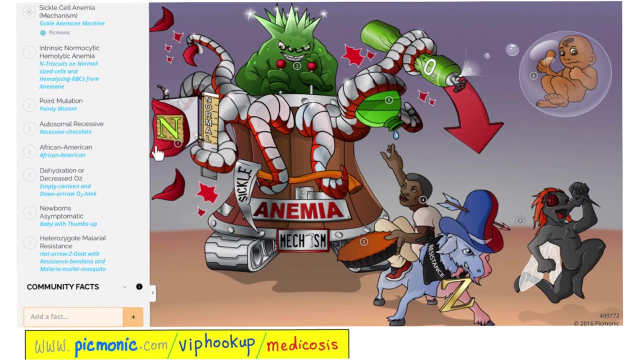 disease. I have a video about this in my hematology playlist. Let's review some facts about sickle cell anemia from Pygmonic Sickle cell disease. You can see the sickle here. It's an intrinsic normocytic normochromic anemia in triscus on a normal sized red blood cell. And look at the. 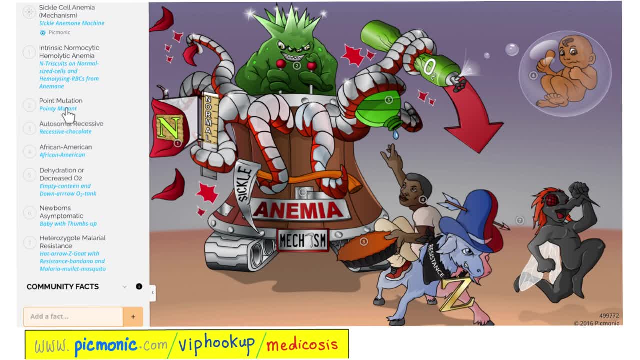 destruction. That's hemolysis. right there, It's due to a point mutation. Here is a pointy mutant that happens to be autosomal recessive. This is that recessive Reese's chocolate. This disease is more common in African-Americans. The hemoglobin S or the. 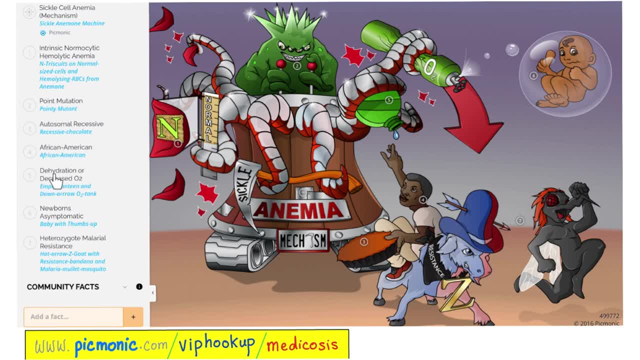 sickled. hemoglobin is very sensitive to hypoxia And that's why anytime I'm dehydrated or anytime I have hypoxia, the cells will start to sickle. Here is the low oxygen. Newborns are usually asymptomatic, But as they grow older they can start to suffer from symptoms: Sickle cell disease. 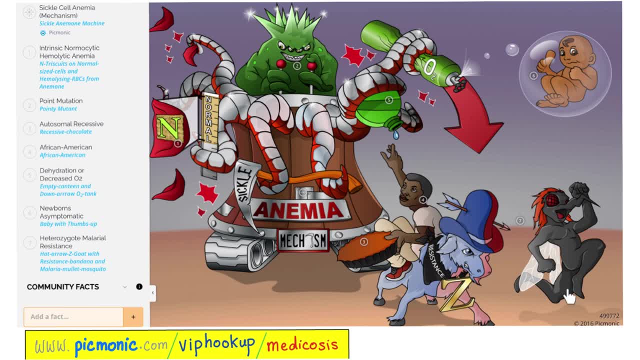 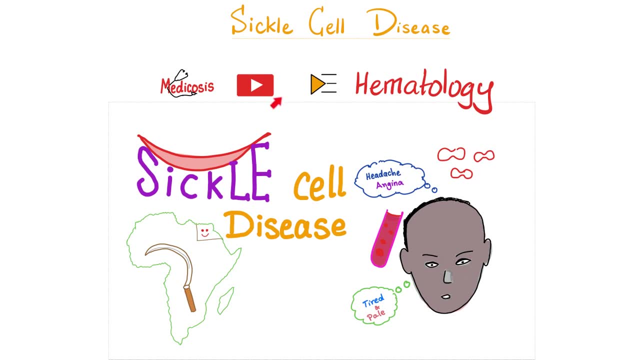 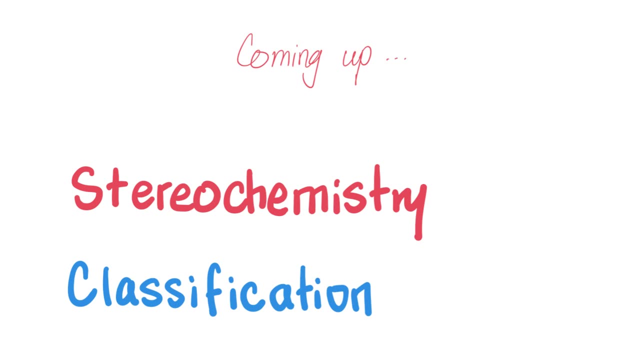 will give you resistance against malaria. Here is the malaria female anopheles mosquito running away. If you want to learn more about sickle cell disease, I have many videos about it in my hematology playlist Coming up. in the next video we'll talk about stereochemistry. What does it mean to rotate around the plane? polarized light. 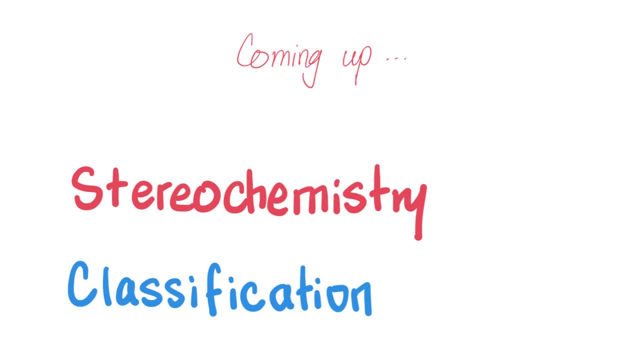 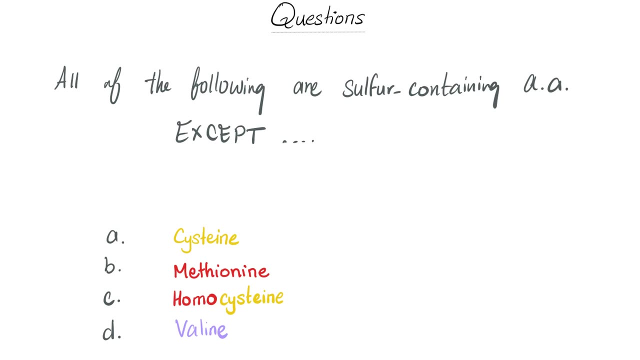 You can rotate to the left, called levo, and you can rotate to the right, called dextro. We'll also talk about classifications of these doozy amino acids. Question of the day is here. Try to answer it and you'll find the correct answer in the next video.